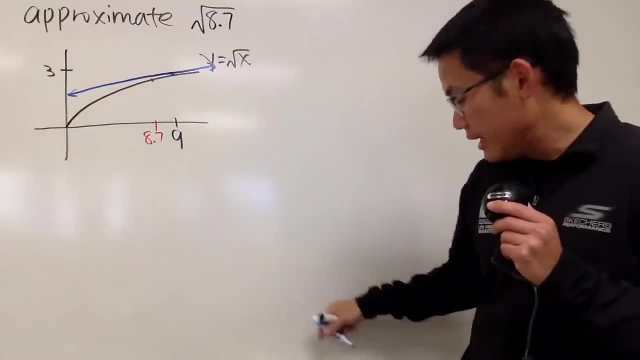 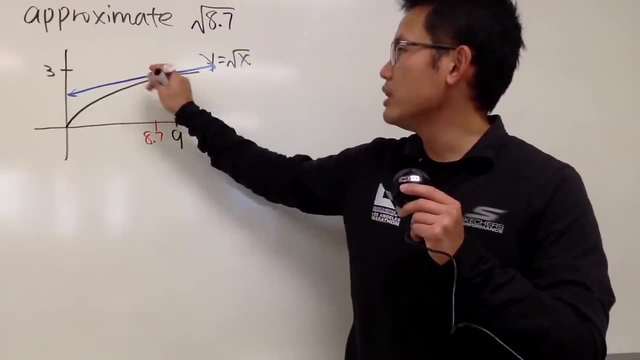 So this is meant to be the tangent line And I'm going to draw a line tangent to square root of x and instead of putting down 8.7 to square root, I am going to put down 8.7 to the tangent line. 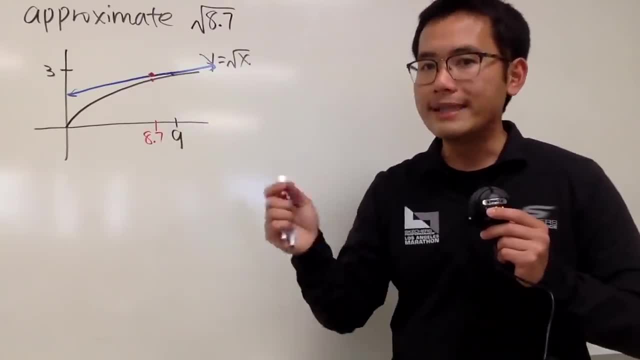 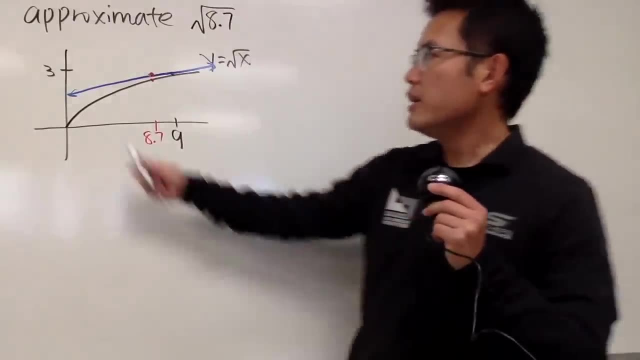 equation. because the tangent line equation has the form: y is equal to mx plus b, And it's really easy to multiply, divide and subtract right. So that's the idea. Therefore, let's go ahead and find the equation of tangent line first. So what we need is two things. First of all, 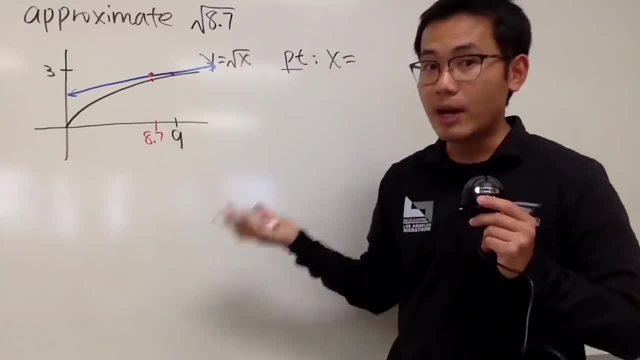 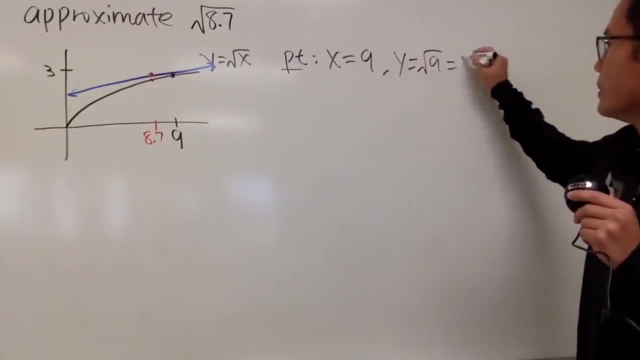 point, of course, x is equal to 9.. And this is like my original. this is what we know. So that's the original right. When x is 9,, y is equal to square root of 9,, which is just going to be 3.. So the point is 9, 3.. And that's x1, y1,. right Now let's go. 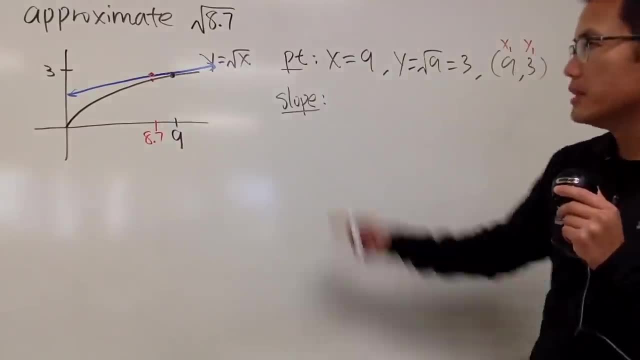 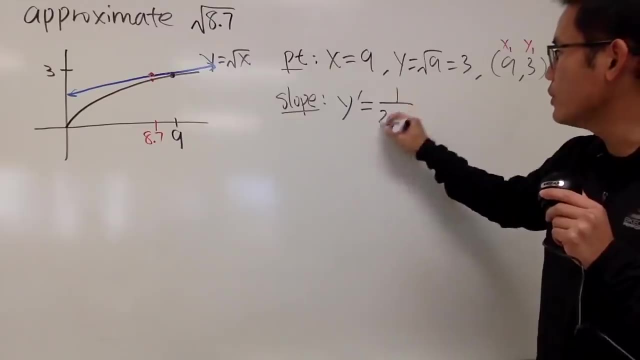 ahead and find the slope. Well, for the slope it's, of course, just the derivative of that Derivative of square root of x is 1 over 2 square root of x, like this, And again we are going to. 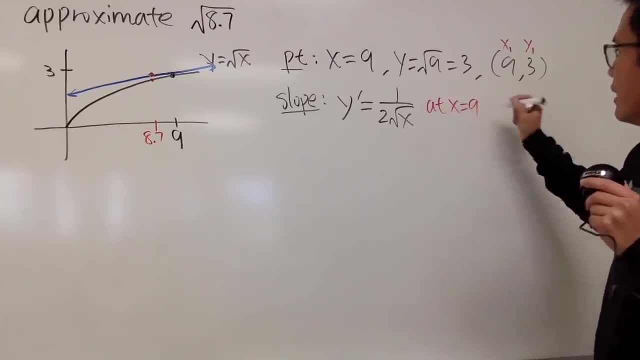 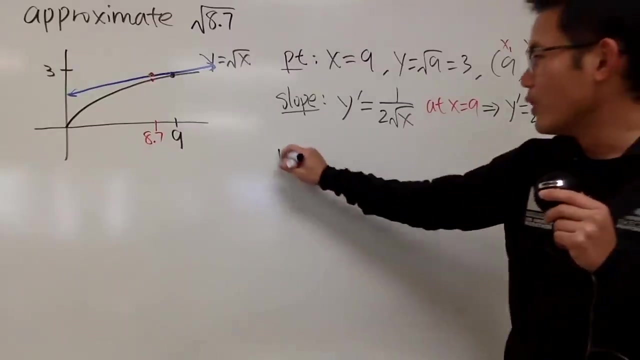 plug in at x Equals 9.. So we are looking at this as y prime equals 1 over 2, square root of 9.. Work this out. That's of course 1 over 6. And this is the slope. And then we can use, of course, the. 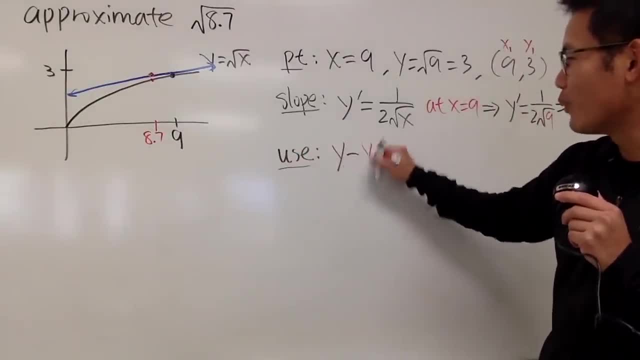 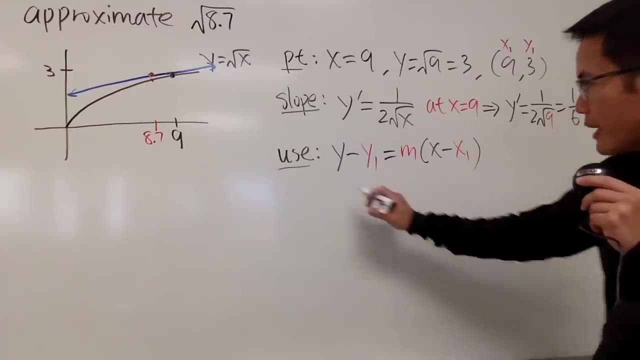 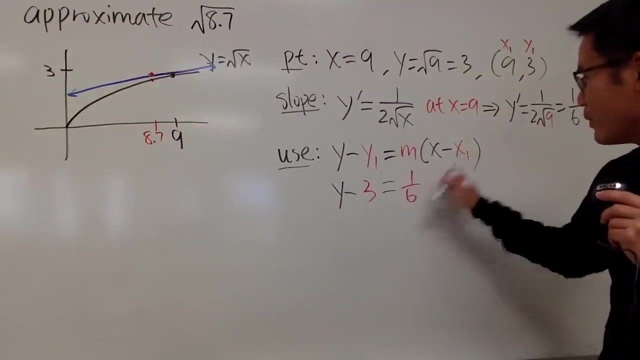 Google equation, The point slope form right: y minus y1, that's equal to m times x minus x1.. And drawing everything: Okay: y minus y1,, which is 3.. m is 1 over 6.. And then we have x minus x1,, which is 9.. So that's what we have, right. 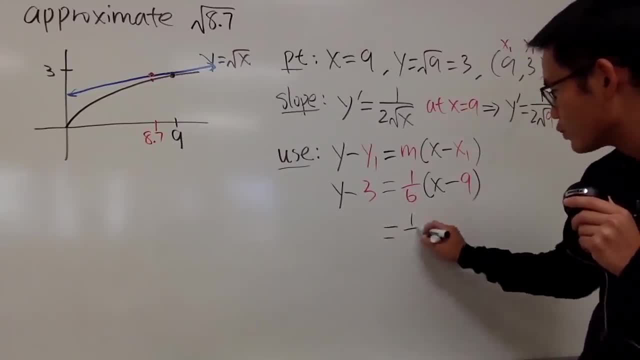 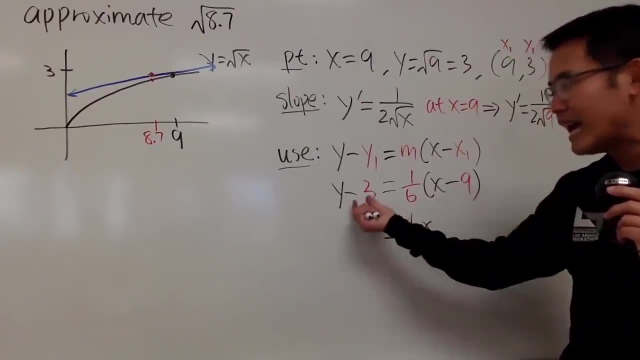 And now let's do this in our head: This times that is of course 1 over 6x. This times that is going to be negative 3 over 2.. But then I have to add the 3 on both sides: Negative 3 over 2. 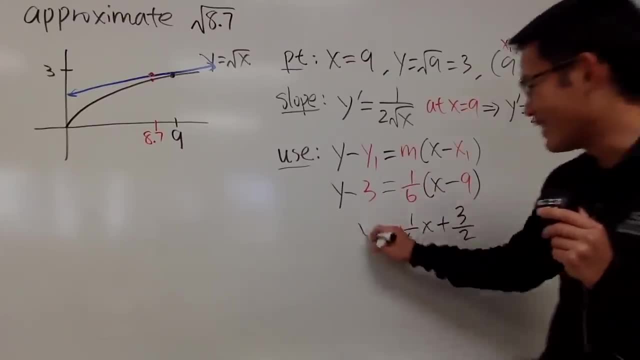 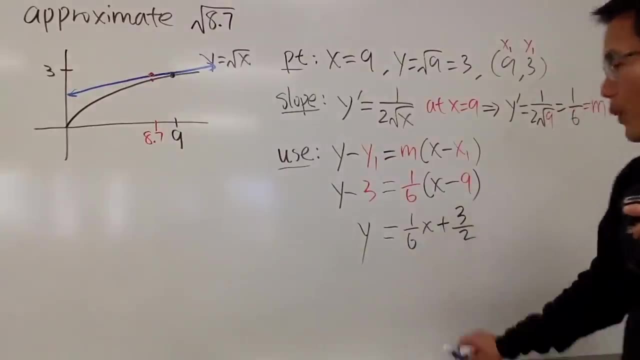 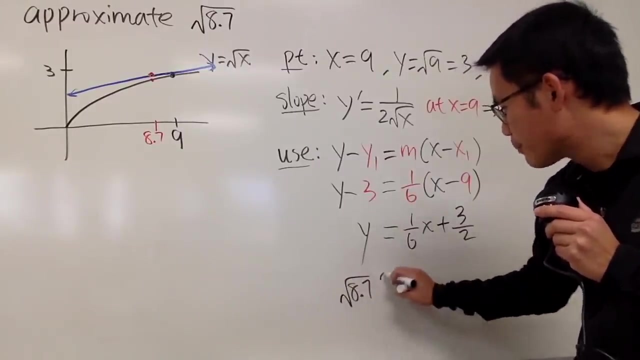 plus 6 over 2.. We add 3 over 2.. Just work that out on your own. All that good stuff, That's pretty much the equation of the tangent line. Then what we can say is square root of 8.7.. I'll just put this down here for you guys. It's approximately equal to 1 over 6. And I'm 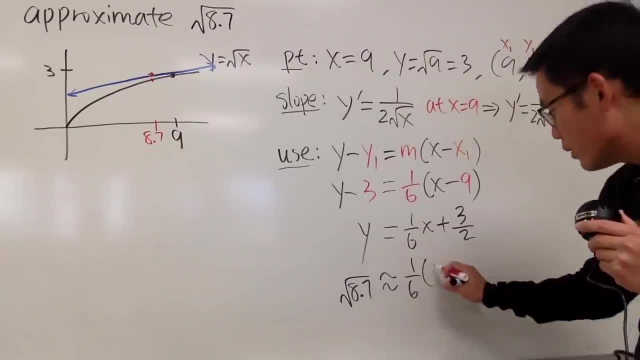 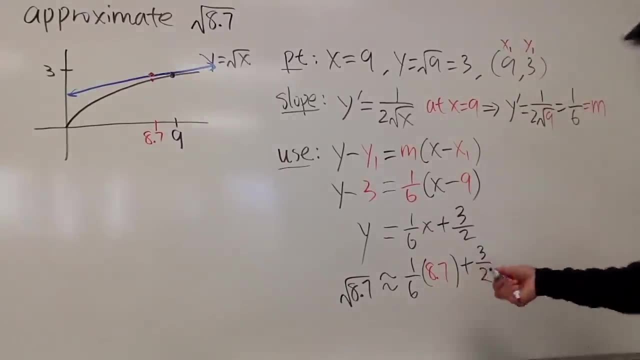 just going to put in the x value to be 8.7 right here, And I will add 3 over 2 after that. Well, just to show you, I can do this with our calculator. Of course, we can do this by long. 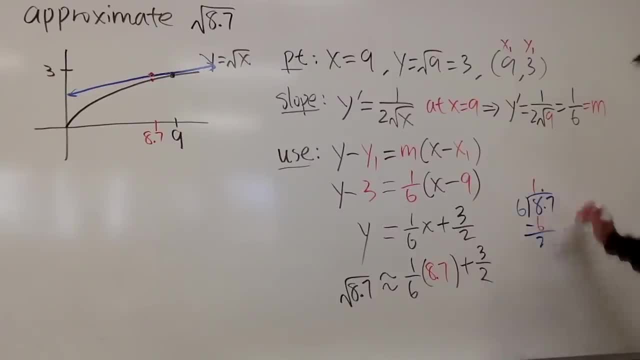 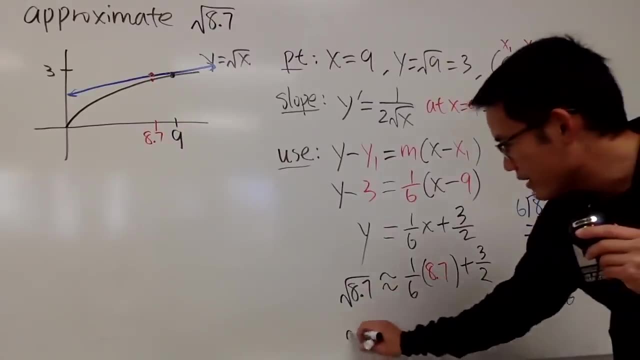 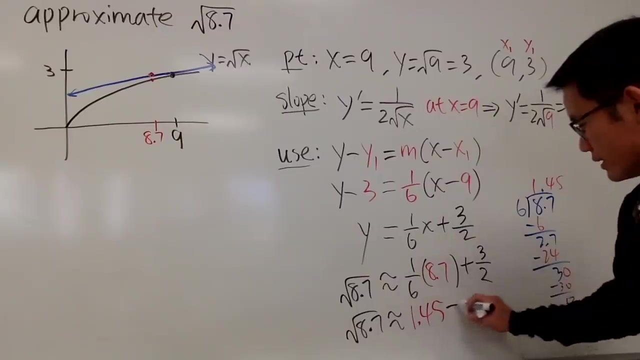 division. Good stuff, yeah, So we are saying square root of 8.7 is approximately equal to 1.45, plus of course, this is 1.5.. That's right, Of course we're saying square root of 8.7.. 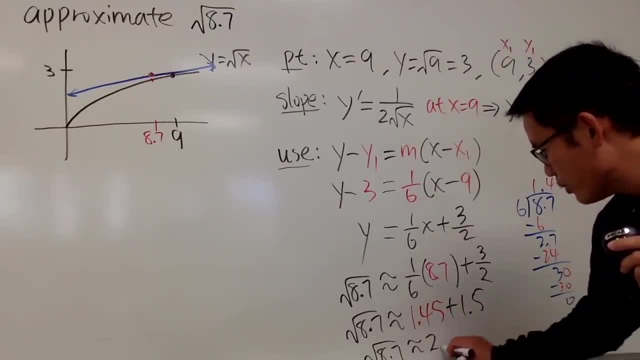 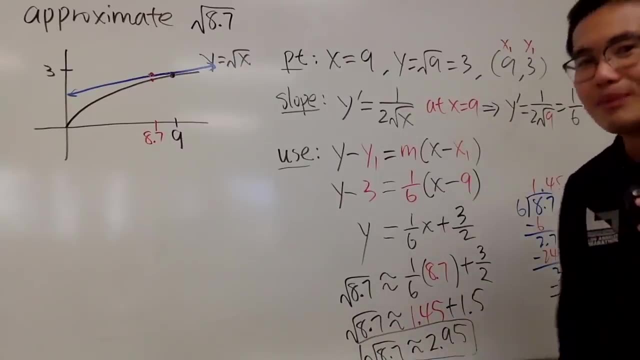 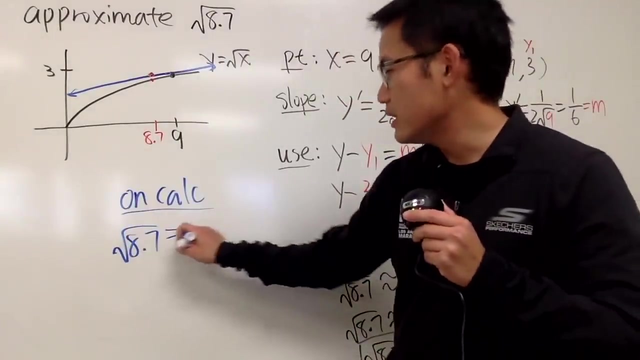 This right here is approximately equal to 2.95.. So that's how you can use the tangent line approximation to help us out. Well, I will tell you, guys, though this right here on the calculator, it's going to tell you that's equal. 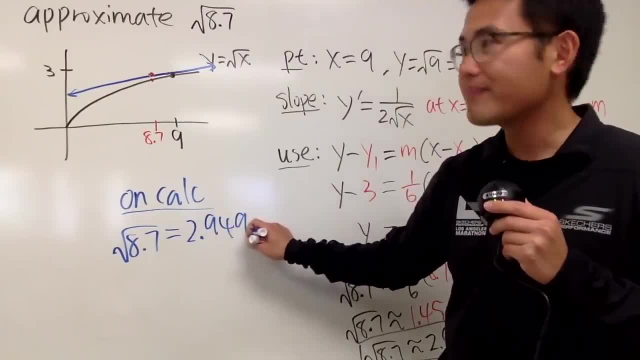 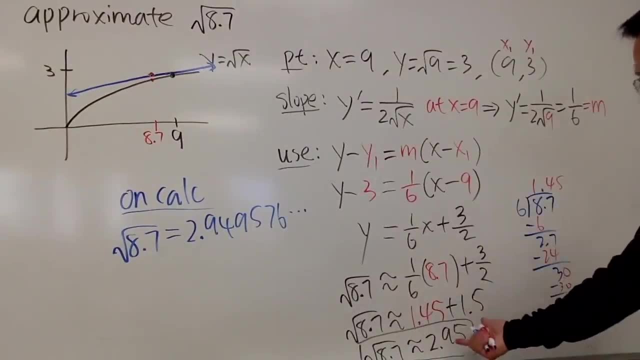 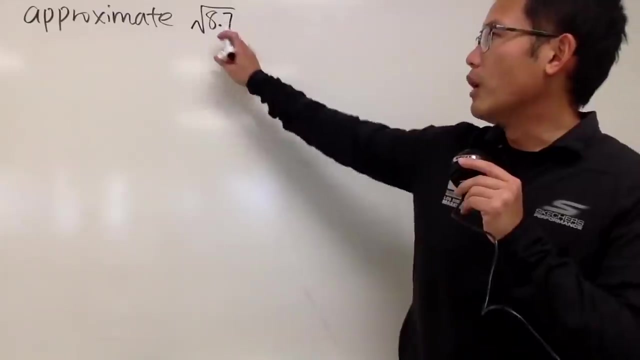 to 2.949.. 5,, 7,, 6, and so on, so on, so on. It's irrational, of course. As you can see, our approximation is very close to the calculator's answer. Of course we don't know. square root of 8.7.. 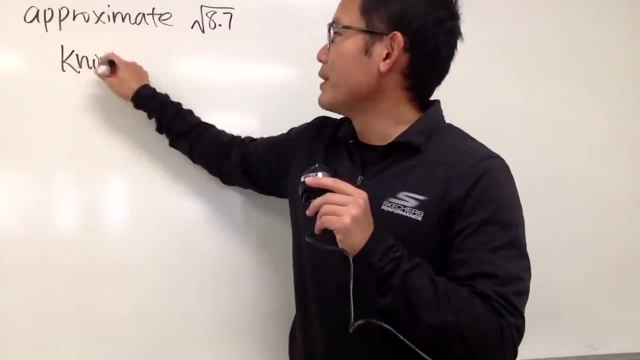 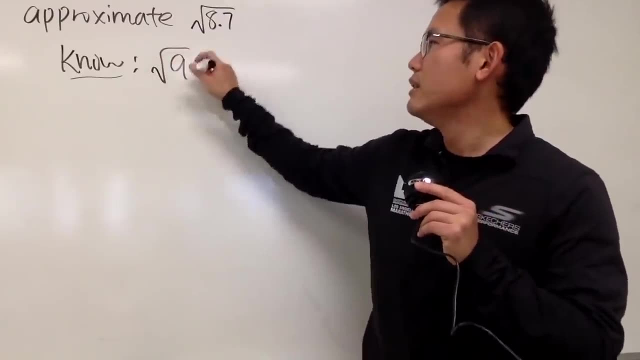 But we do know it's the following: Well, let me write it down right here for you guys: We know that when we have square root of 9, this right here is nicely equal to 3, right? And the reason I picked 9 is: well, of course, 9 is pretty close to 8.7.. 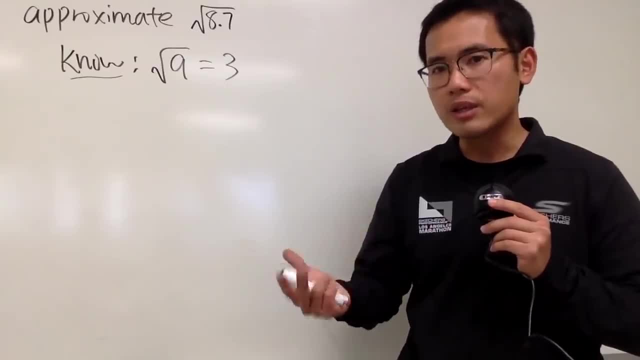 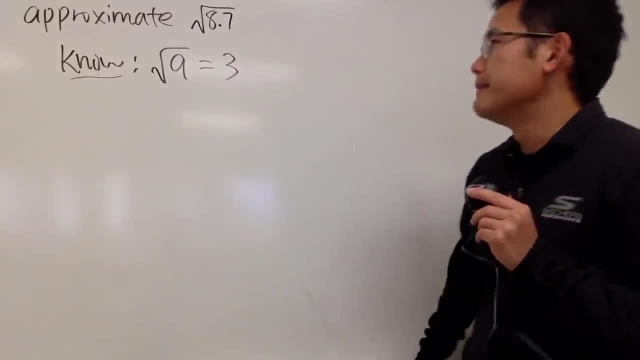 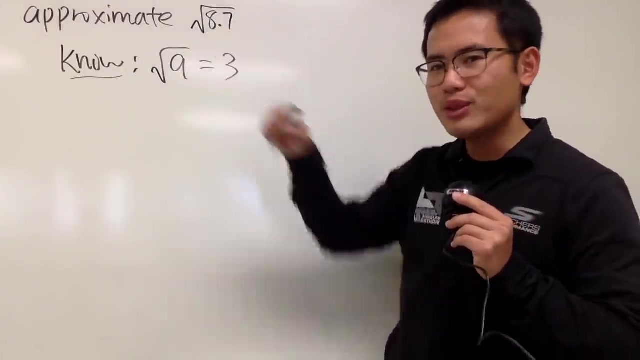 This right here is my original point, And in calculus we have to think about functions. In our situation, we are, of course, talking about square root of x. Hmm, Okay, So the x-value right here is 9.. And the new value is 8.7.. So you can see that we have the 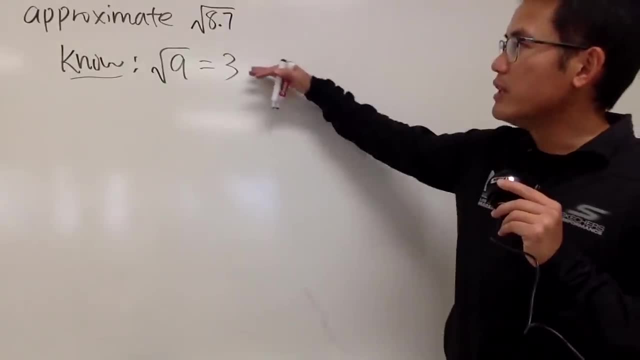 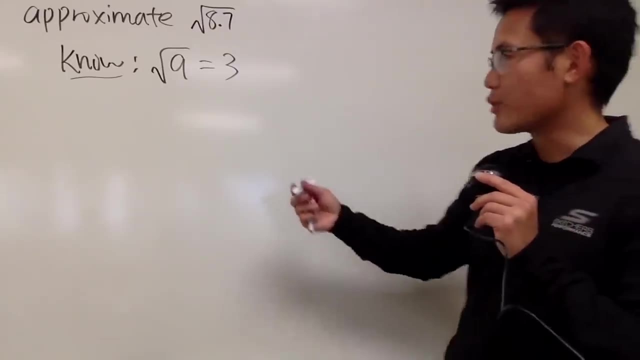 difference in the x-value. Well, if we can figure out the difference in the y-value, we can get the approximation done. That's pretty much it right, And actually let me write this down right here for you guys: Square root of 8.7, this is the y-value on the 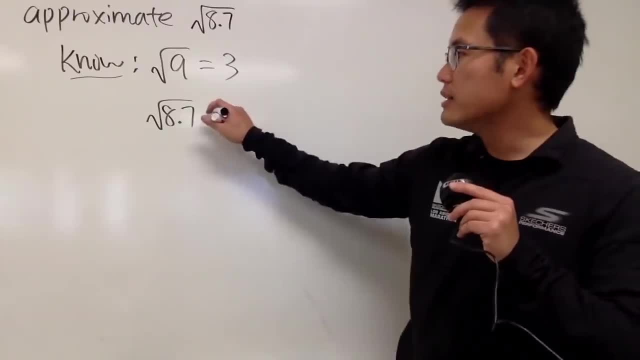 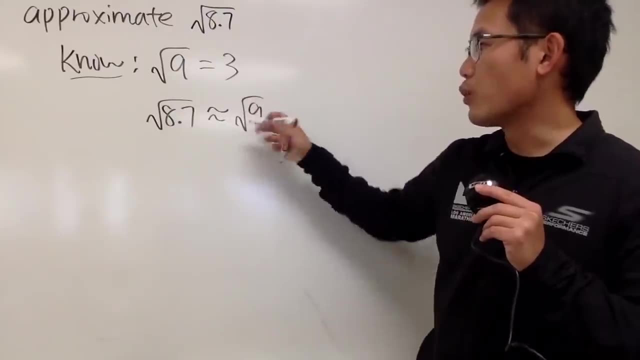 graph of square root of x. Well, this right here, it's going to be approximately equal to the original y-value. Now, if we know, name this square root of 9, which is of course 3,, but I need to figure out the. 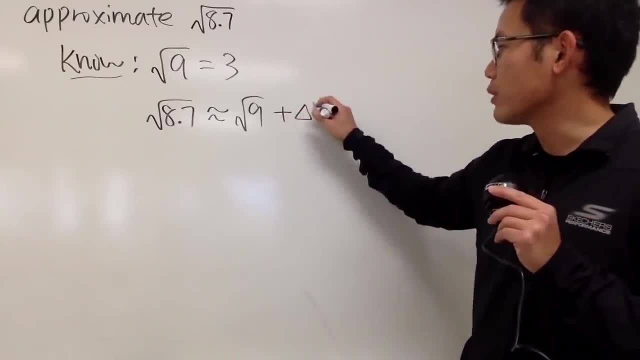 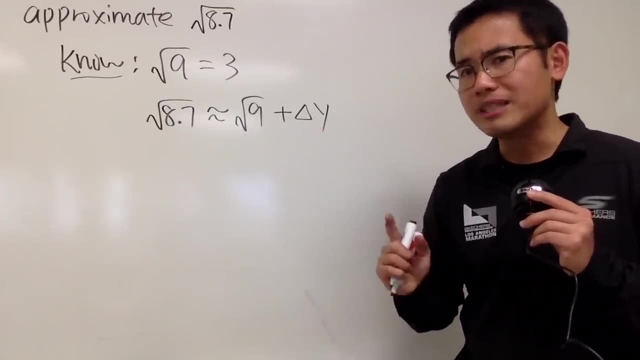 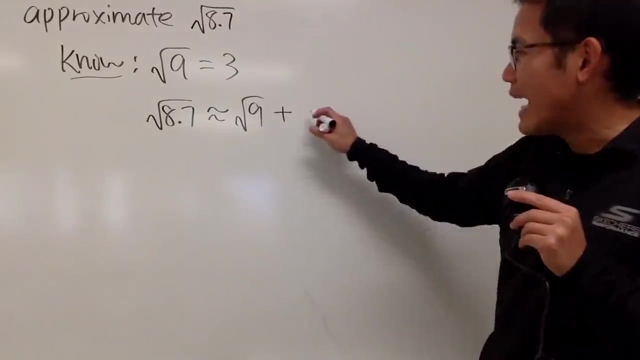 change in the y-value, right? So I'll just put down plus delta y like this: This right here means the exact change in the y-value, But the problem is that we cannot compute that nicely with our calculator or whatever. But what I can show you is that though we can add dy for it, because dy 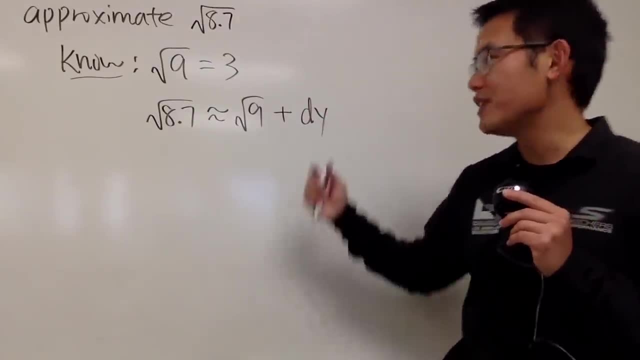 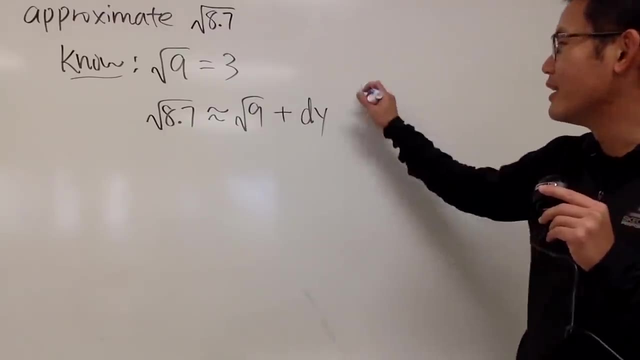 is the approximate change, And we can just use derivative To help us figure this out very nicely. So how can we do that though? Well, have a look right here For dy. first of all, of course, we are talking about y equals square root of x, as I 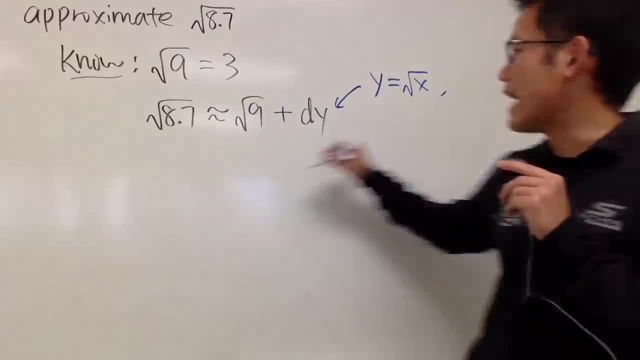 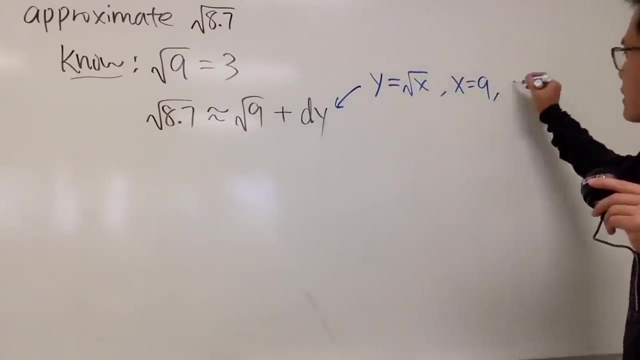 mentioned earlier, And my original x-value is 9, right, Because this is the one that we know. So that's the original And we also have to figure out the change in the x-value. Again, originally is 9,. 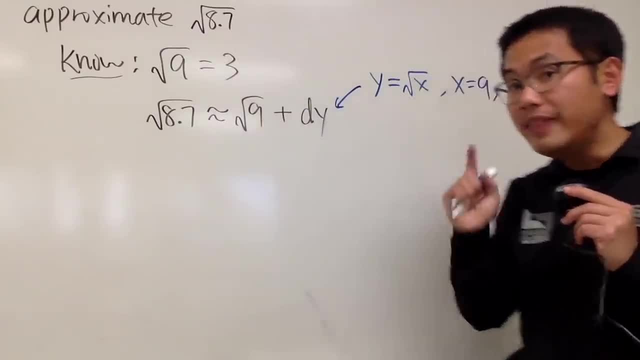 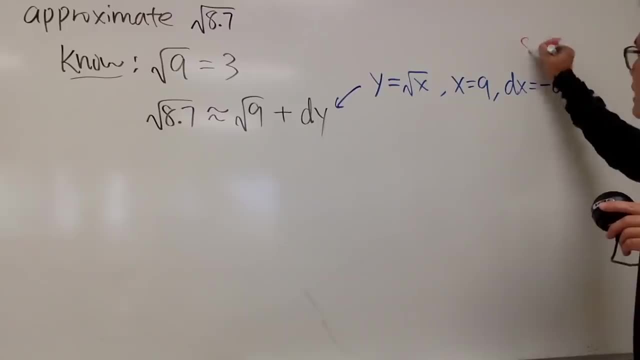 which is 8.7.. That's what we're trying to figure out. So the difference is negative: 0.3.. Again, you always need to use the new value that you're trying to look at, which is 8.7 minus the. 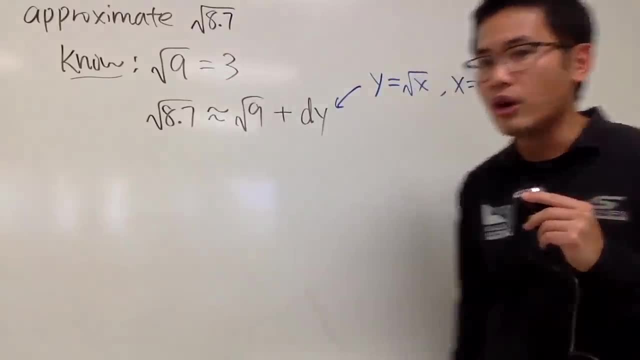 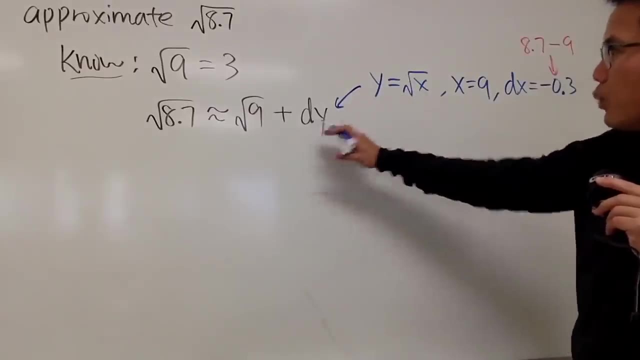 original right. Minus what you know, That's the original. So that's why dx is negative 0.3.. And now we can just do the computation To get the y. of course you differentiate this, but you talk about differential. So you just do dy and that's equal to you do the derivative of. 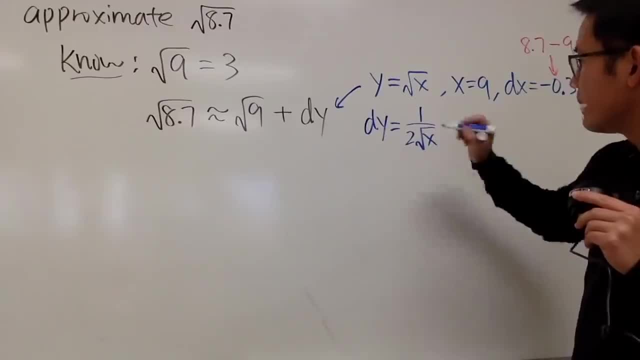 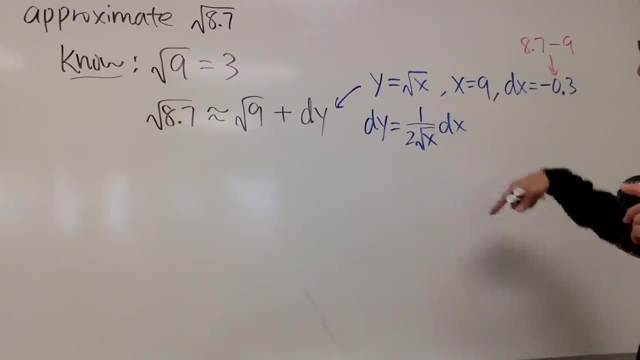 this, which is 1 over 2 square root of x, but we multiply by dx, So that's pretty much it. but we have to then plug in the x-value and also the dx and all that. So dy equals 1 over 2 square root of 9. And the dx is negative, 0.3. that we have to multiply.